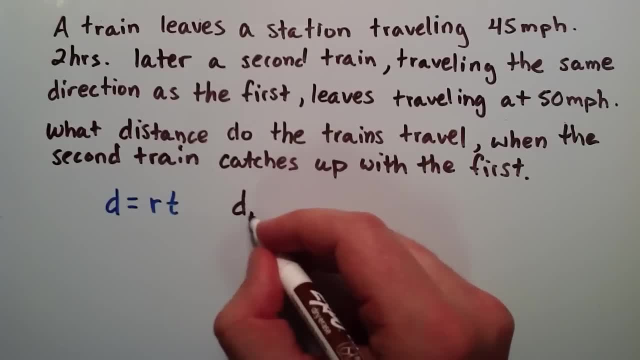 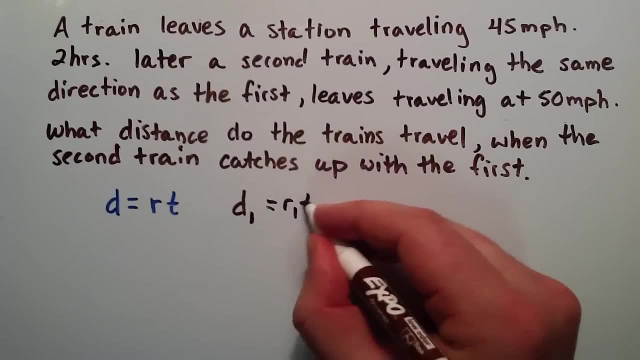 So I'm going to be explicit and say that the distance- d1 is going to be the distance that train 1 travels- Is equal to r1- t1.. So the distance that train 1 travels is equal to the rate that train 1 is traveling multiplied by the time that train 1 has traveled. 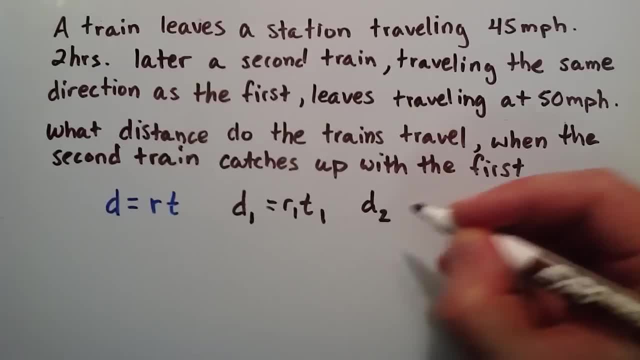 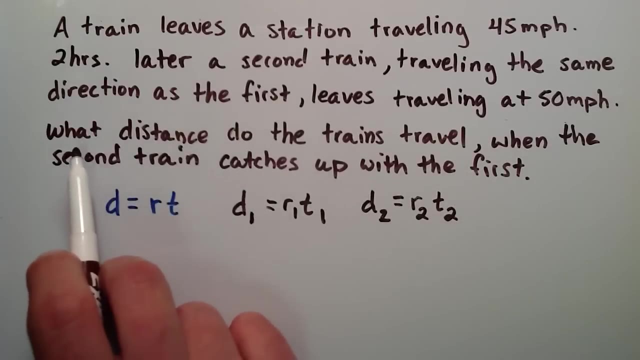 And then we can also say in an explicit form here: d2, the distance train 2 has traveled is equal to the rate that train 2 is traveling multiplied by the time that train 2 has traveled. So When we want to figure out what distance the trains travel when the second train catches up with the first, 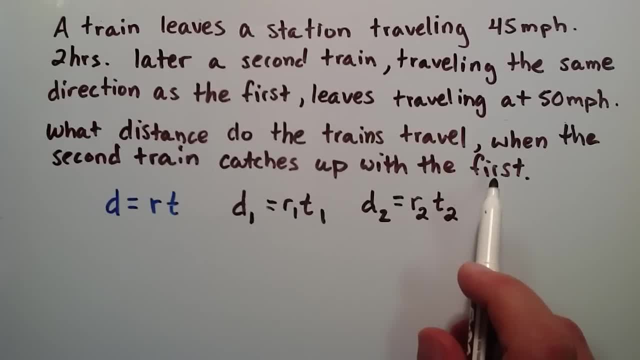 We need to realize that the distance will be the same for both trains at that point, When they're both the same distance from the train station, they've caught up with each other, And so, therefore, at that point in time, the distance train 1 has traveled is equal to the distance the train 2 has traveled. 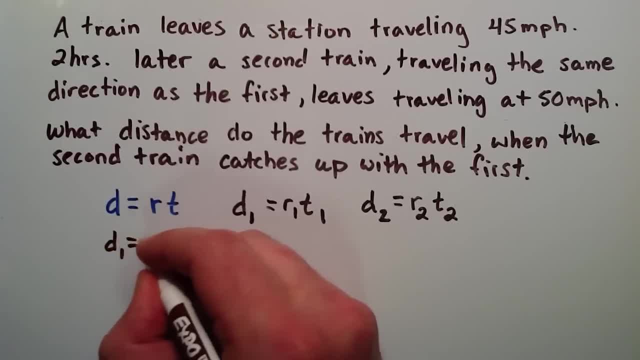 So that's going to be the situation we're looking at. When d1 is equal to d2, is when this happens, And since I explicitly made these statements here, we can simply replace D1 with R1- T1 and D2 with R2- T2.. So let's go ahead and do that now. Instead of D1, we'll write R1- T1.. 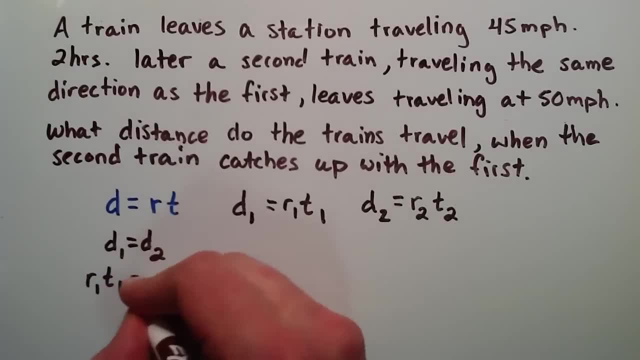 So right here, this changes to R1. T1 is equal to D2, which we said was R2, T2. And we know what R1 is, We know what R2 is. Those were given in the problem, But we need to figure out how we can write these two times with a variable. that kind of can relate. 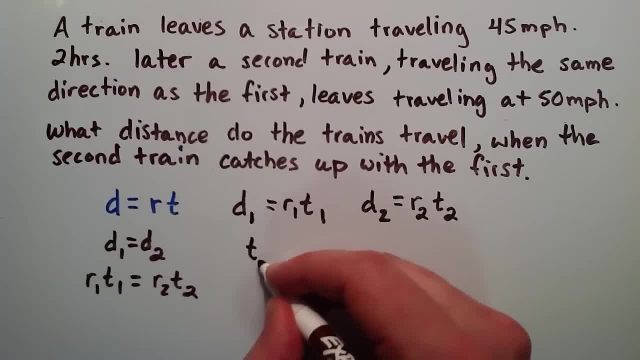 to both. So what we're going to do is we're going to say: let's just pick and say that T1 is going to be equal to X, So X equals the amount of time that train one has traveled, And then we'll 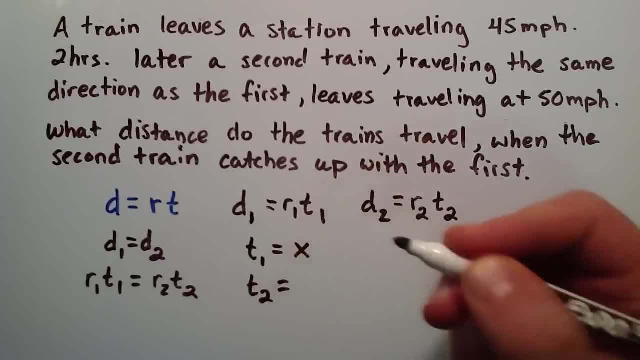 we'll say that T2 is equal to X minus 2.. So why did I choose X minus 2?? Well, train 2 is basically traveling the same amount of time as train 1, that's the X. but then we have to take away the 2 hours that it was at the train station before it took off. So 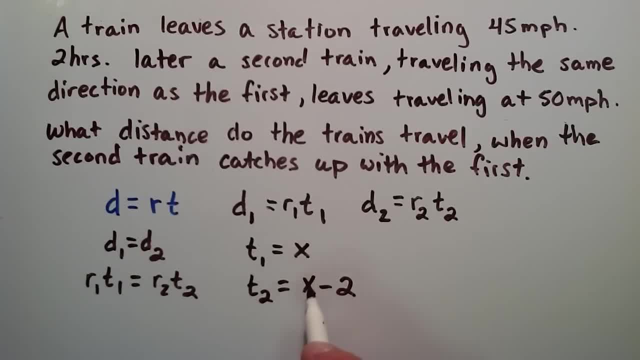 whatever the amount of time that train 1 has traveled, train 2 has traveled 2 hours less. So now let's go ahead and replace these two values where the T's are in this equation here, So this becomes R1, T1, we're saying is X, and that's equal to R2, and T2 is equal. 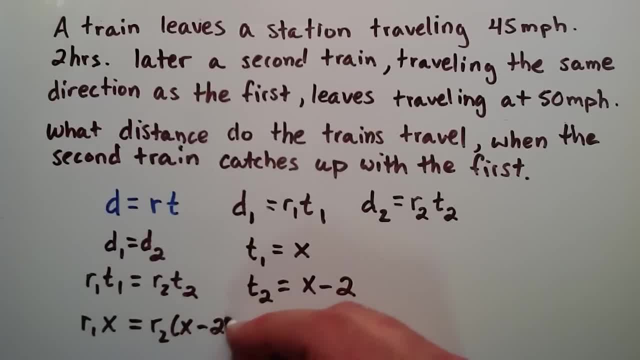 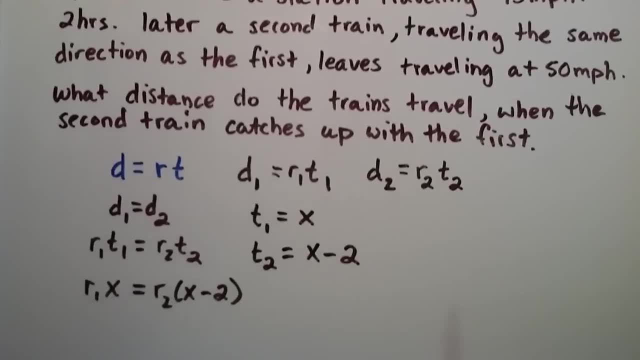 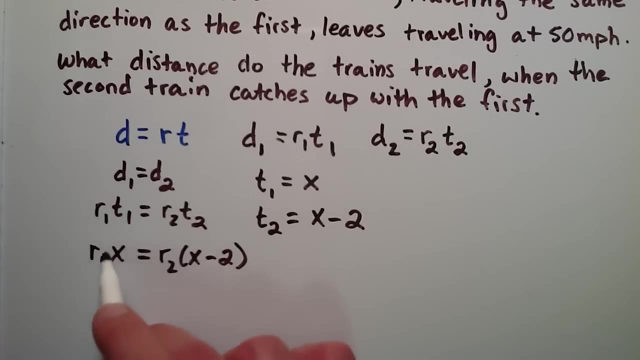 to X minus 2.. And be careful to put these in parentheses here, since we're multiplying R times the entire quantity of T, so the parentheses are important here, And so then we're just basically we're going to plug in the values of R1 and R2.. We said that train 1 was traveling at a rate of 45 miles. 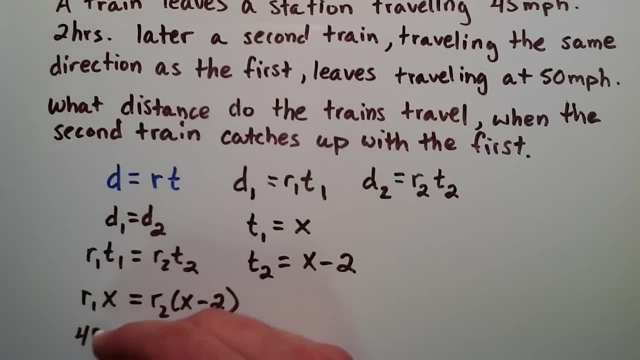 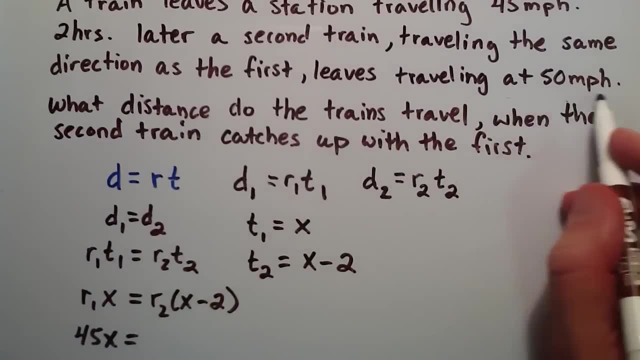 per hour. So we're just going to put the number 45 here for R, So now we have 45X is equal to R2 was the rate of the second train. that was 50 miles per hour, So this becomes 50. 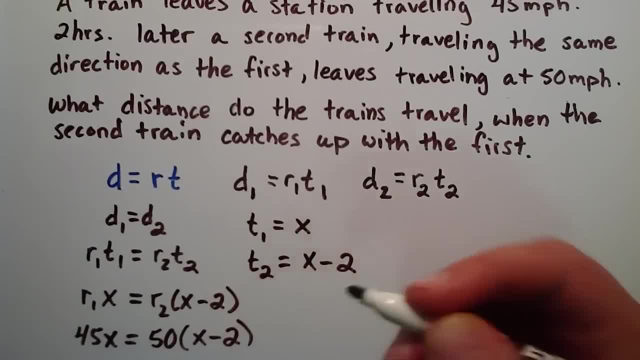 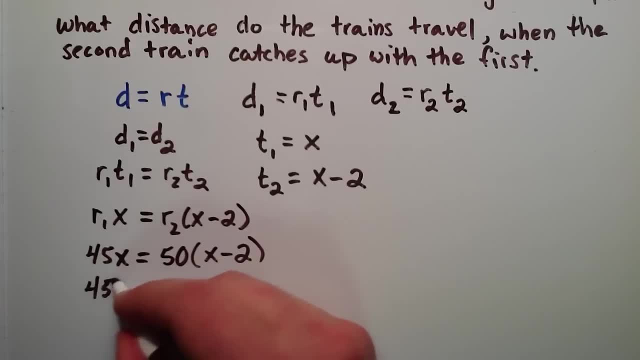 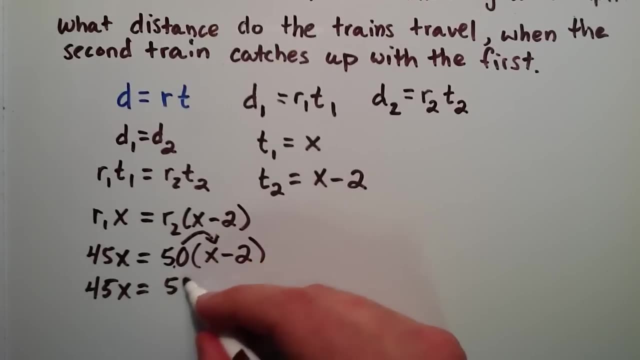 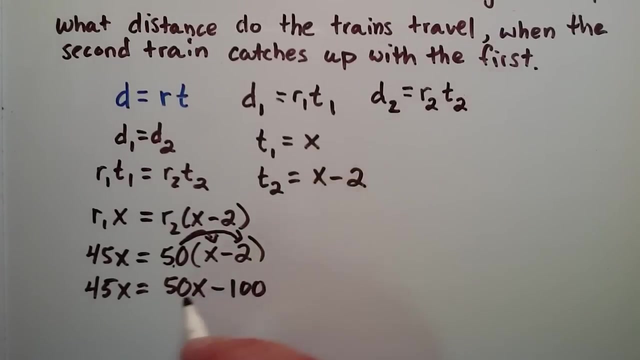 multiplied by the quantity of X minus 2.. So now we've got an algebraic equation here to solve, So we'll just rewrite the 45X here, And then that's equal to 50 distributed into the parentheses here. 50 times X is 50X minus 50 times 2 is 100. And then I'm going to subtract 50X from. 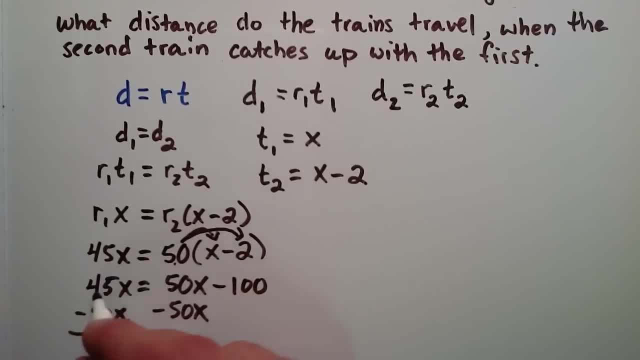 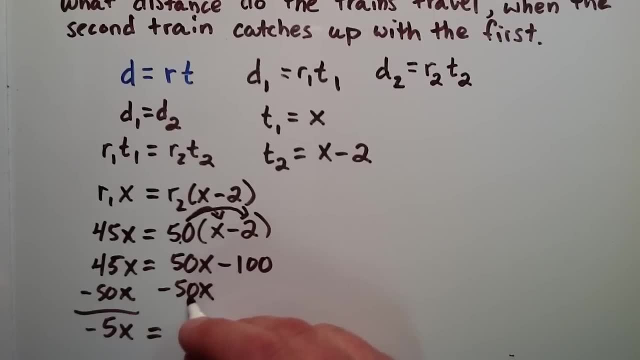 both sides, And 45X minus 50X gives us a negative 5X, And 50X minus 50X gives us a negative 5X, And 50X is 0, leaving us with negative 100.. So then, just dividing each side. 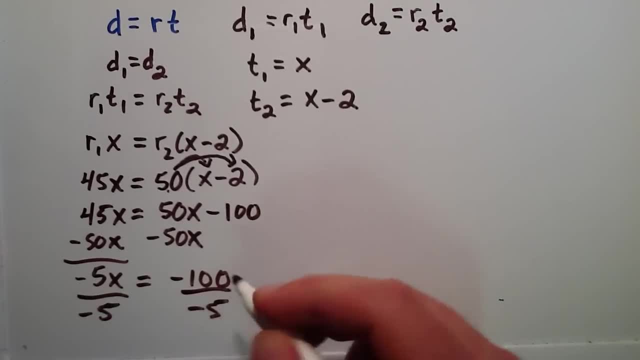 by a negative 5. here The negative 5 and the negative 5 cancel. Negative and negative cancel. So then we just have: X is equal to 100 divided by 5.. 100 divided by 5 is equal to 20.. So 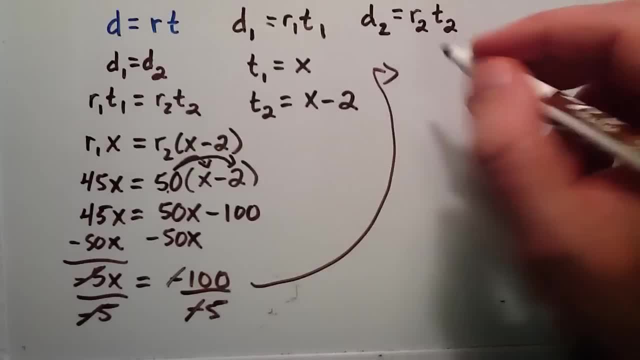 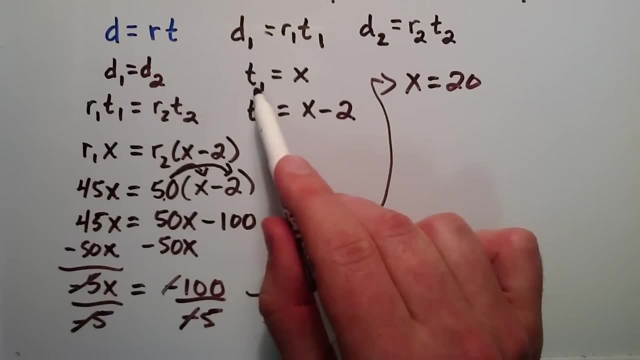 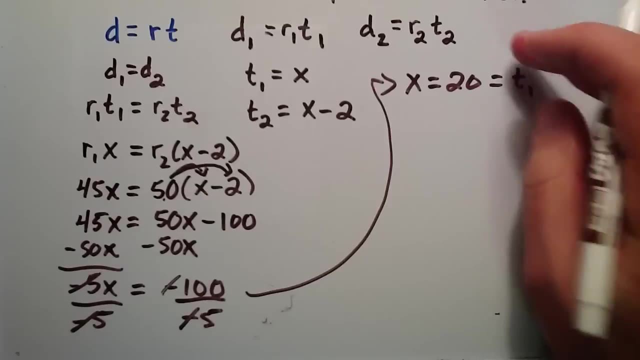 let me just probably rewrite this here so it's a little more clear. So X is equal to 20.. And we said that X was equal to the amount of time that train 1 has traveled- T1. So that means that we have the total amount of time that train 1 has traveled. Let's go ahead. 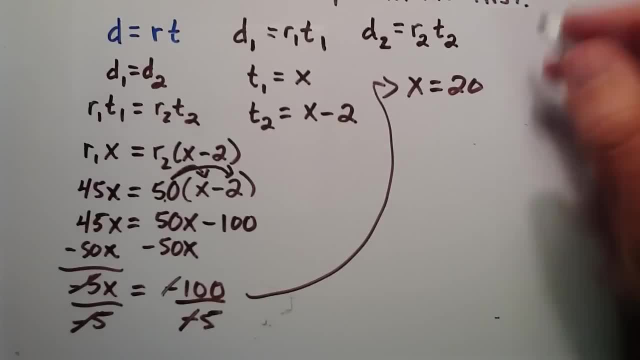 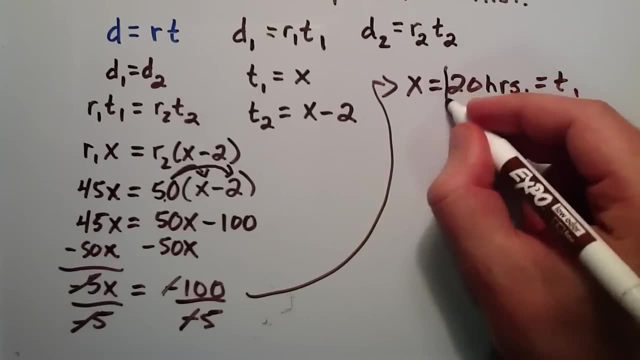 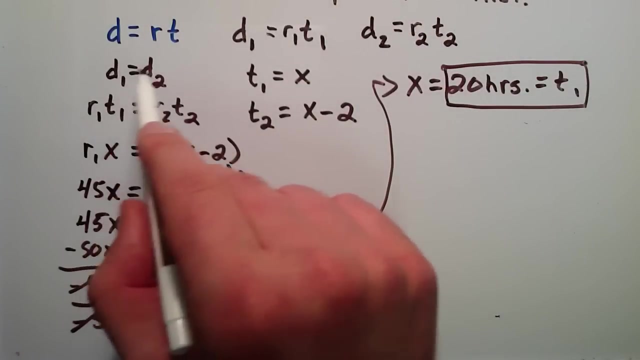 and put hours there. so it's clear: Since we're dealing with miles per hour, this will be 20 hours. That is equal to the time that train 1 has traveled when the two trains catch up. And we know that because we set the distances equal to each other, So we know that the trains 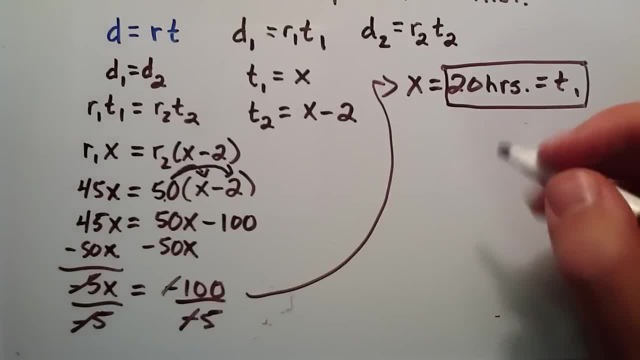 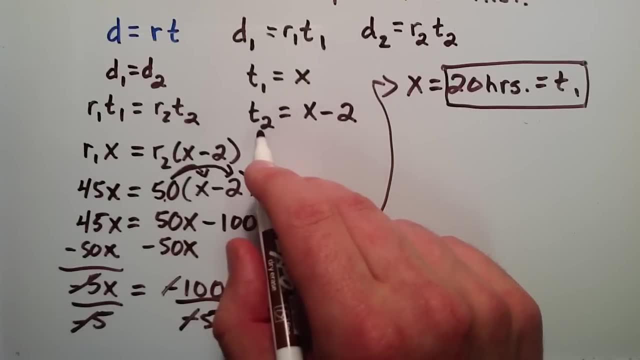 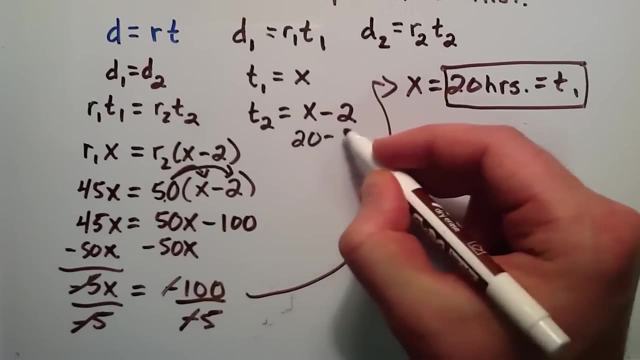 are at the same distance When train 1 has traveled 20 hours. So what about train 2? How much time has it traveled to get to that distance? Well, train 2 has traveled the same amount of hours minus the two hours that it was stuck at the train station. So this would end up just being 20 minus 2.. 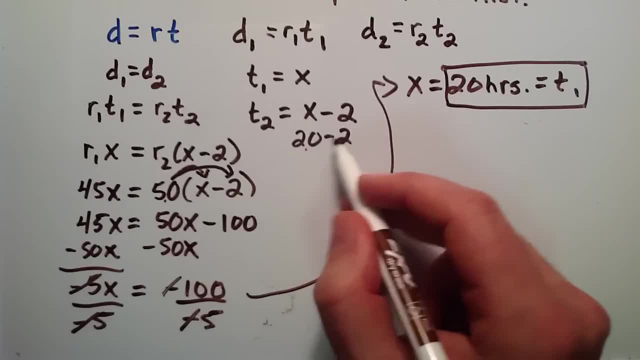 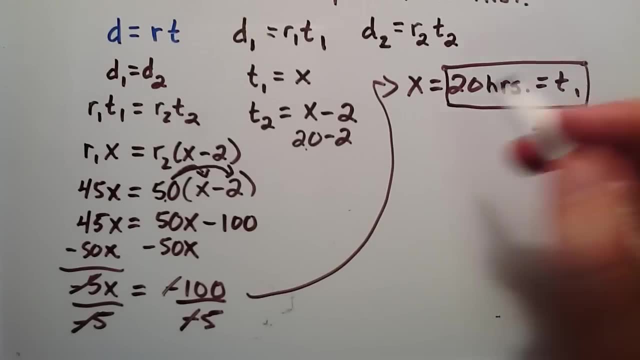 20 hours minus the two hours that it waited would be 18.. 20 minus 2 is 18.. So the time that train 2 has traveled to get to the distance where train 2 catches up to train 1 is equal to 18 hours. So train 2 has traveled 18 years as well. 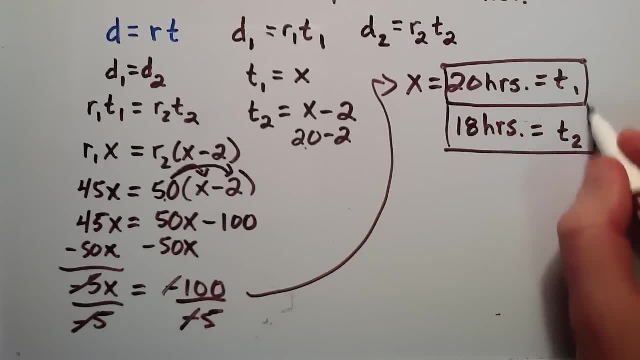 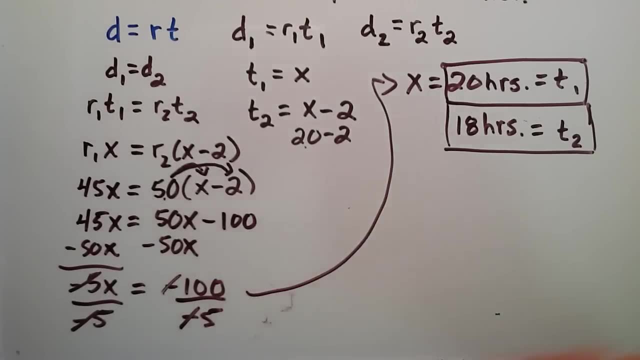 So train 2 has traveled 18 hours, minus the two trains, to get to train 1.. So train two has traveled 18 hours as well. So now we just need to figure out what distance the two trains have traveled to have train 2 catch up to train 1.. So we can simply just 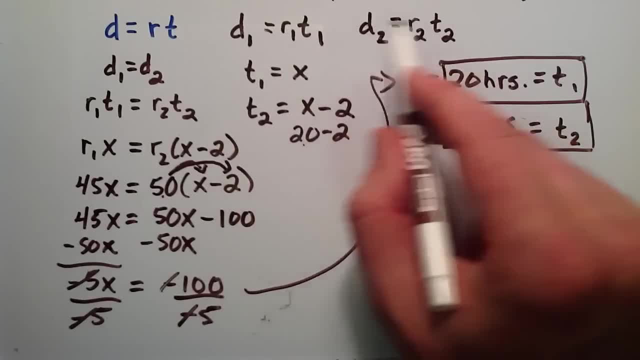 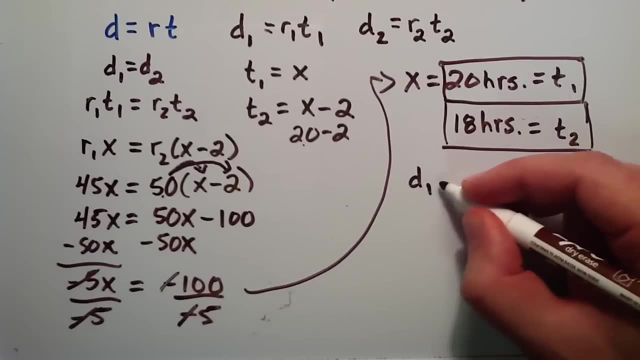 plug into either one of these two equations to find that. so let's go ahead and do both, so that do they're both the same number, So distance when they catch up D1.. Since we'll find the distance that D1 equals 10, now we 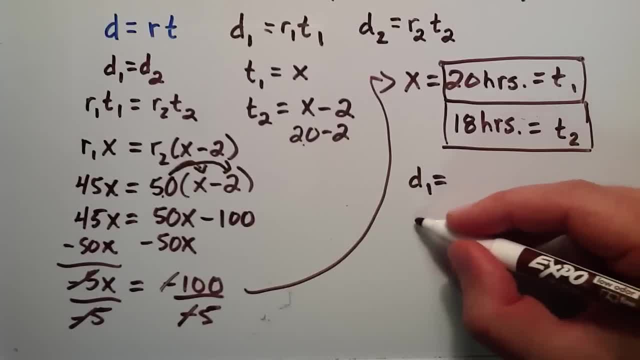 can then use both equals. we find the distance when they catch up D1 is equal to 3.. D willなので you have the distance to hunt trains up, Since we're getting the distance that spin D2.. Then we can do it two different ways here. 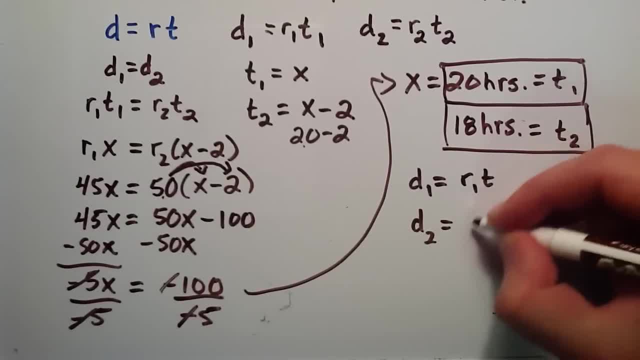 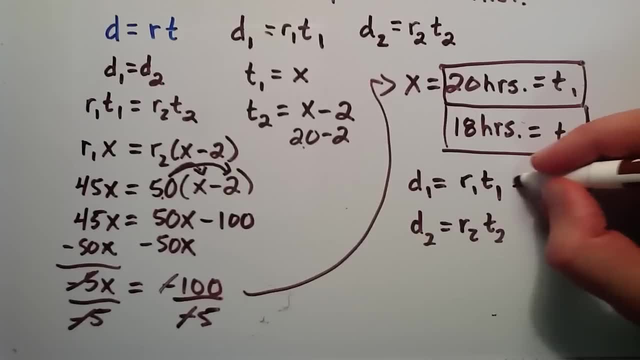 So D1 is going to be equal to R1- T1 and D2 is R2- T2.. So R1 is the rate that train 1 is traveling, which was 45 miles per hour. T1 was the time that train 1 had. 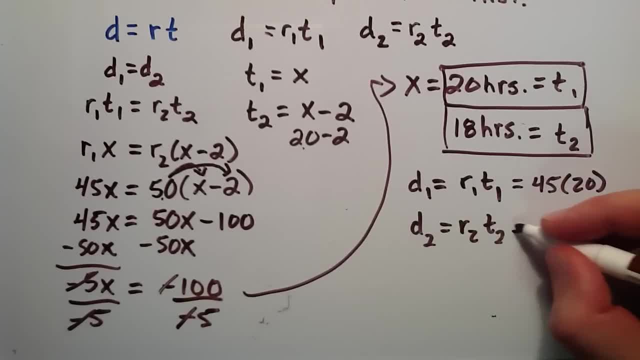 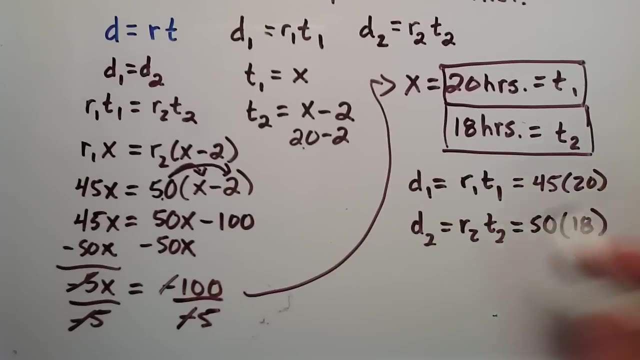 traveled and that's 20 hours. R2 is the rate that train 2 has traveled, which was 50 miles per hour. T2, the time that train 2 has traveled- 18 hours- And we find that the distance where.